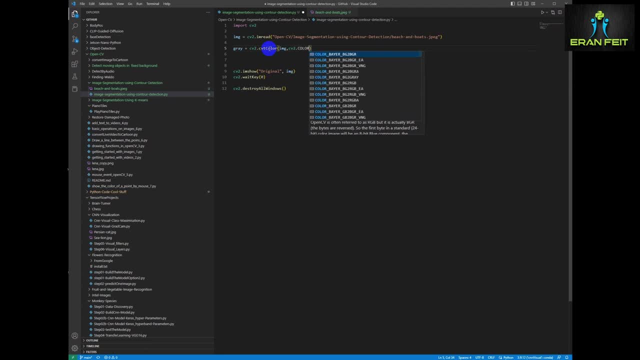 color- The OpenCV's CV2 color- and convert it to gray scale. The next step is doing threshold in order to find the specific gray value and emphasize our part of the image. So let's try the average value of the grayscale in our specific image. 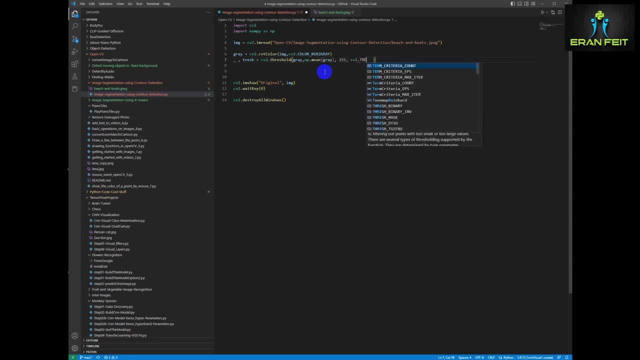 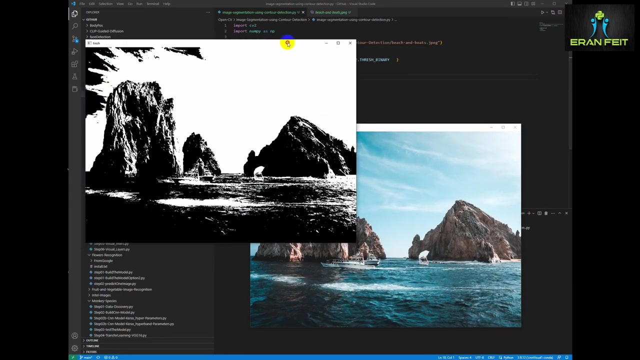 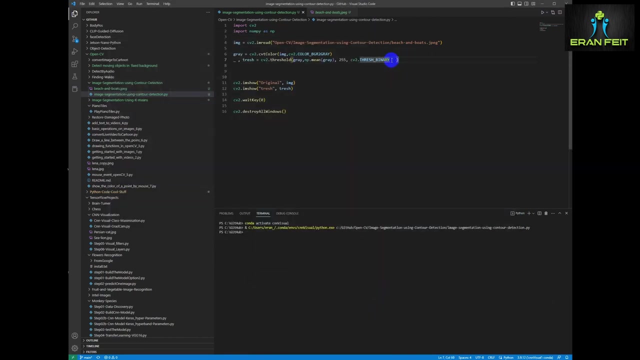 So we will use the numpy mean function and we will send our gray image and we will do the thresholds. Let's show the result. So, as you can see, the mountains are black And the background is black. It's white. So we need to invert it. it should be upside down. 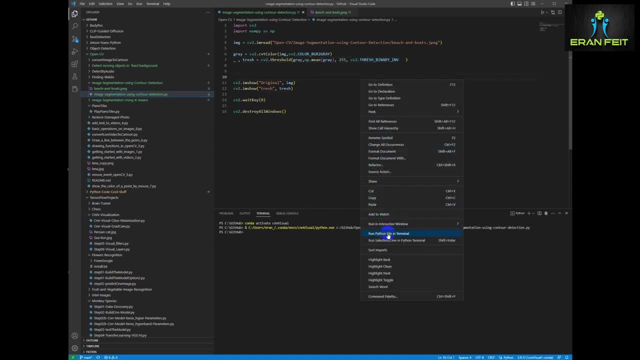 So we will add the fresh binary INV argument and let's run it again. Okay, now it's better And let's continue to the next step. Now we would like to find the contour around these mountains, And this will be the part that we would like to segment. 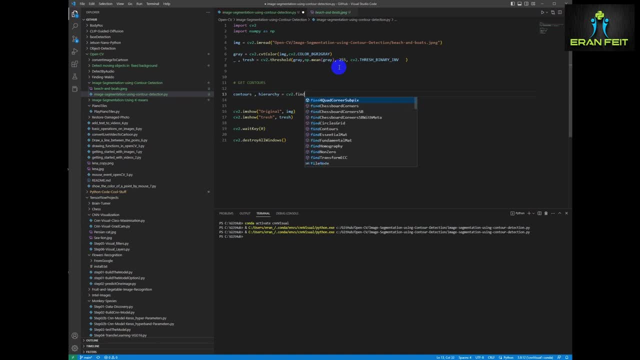 From our image. So let's use the function find contours. We will send our fresh grayscale image, The cv2 rtr list and, as change approx, simple. Let's see how it works. Let's see how many contours, maybe how many types of contours, we have. 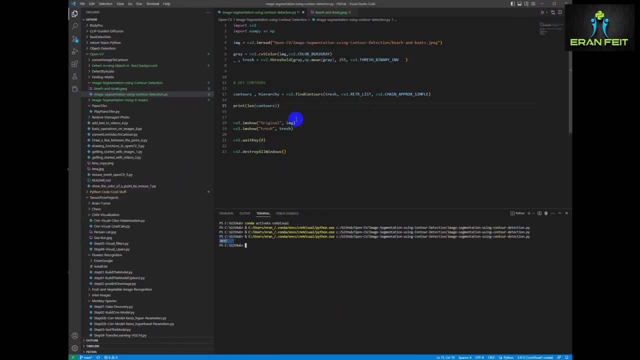 So basically a lot more than 3,000.. Let's try to reduce the number of relevant contours. So we will sort the contours, Let's see. Okay, Let's do it again. So let's see how many contours we have. 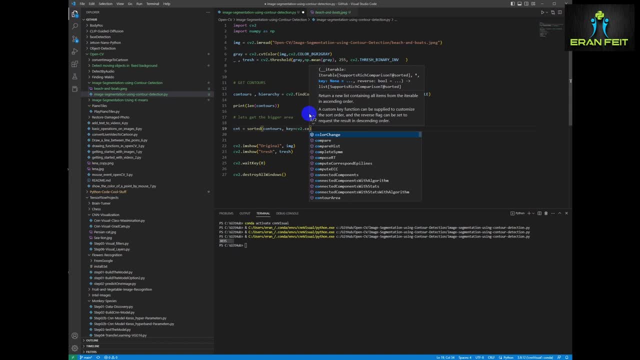 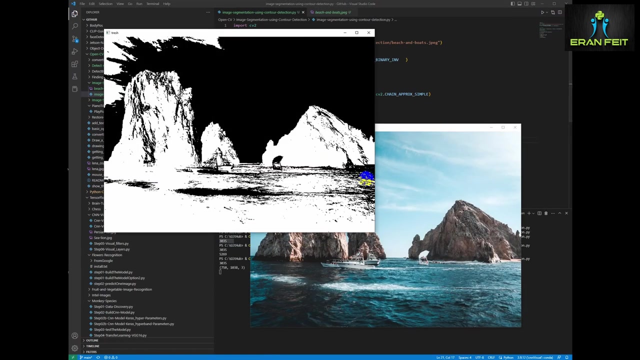 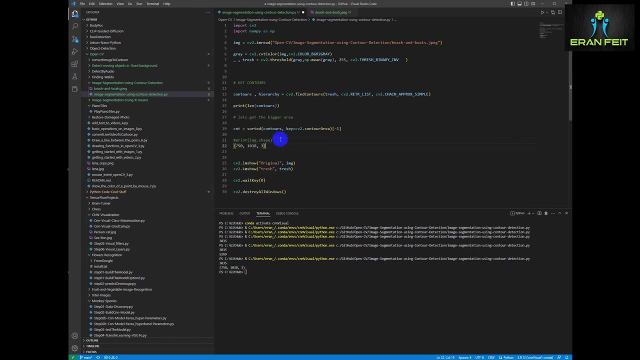 How many contours do we have? so the bigger ones will be the first in our, in our array, and we will try to take the last one. okay, this is the shape of our image it will be relevant to for the next step. Now let's create a mask of zeros based on this shape. so this mask. 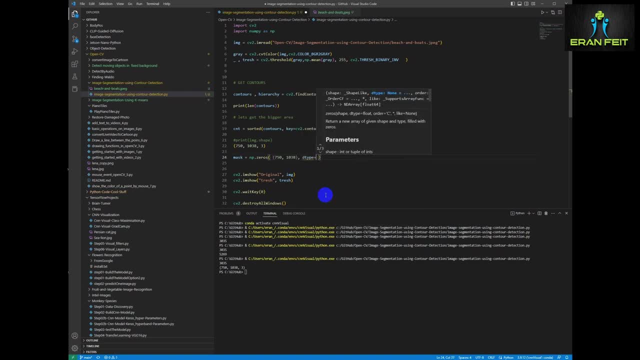 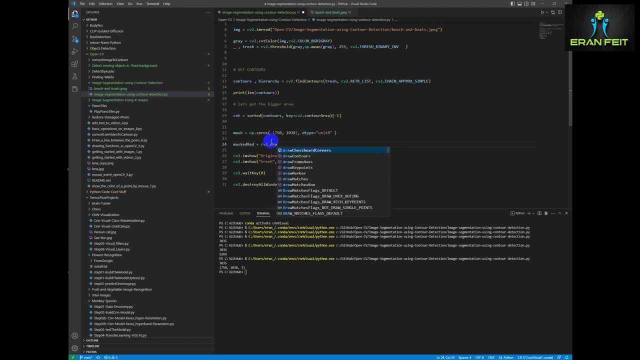 will be the same shape of our original image. Now let's create a, a mask, a on the the red channel. let's see if it's relevant to our process, like a trial, trial and error let's get. let's try to retrieve only the, the red channel and to display it. maybe it will. 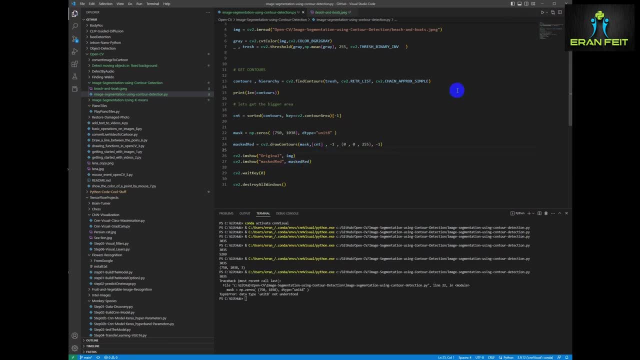 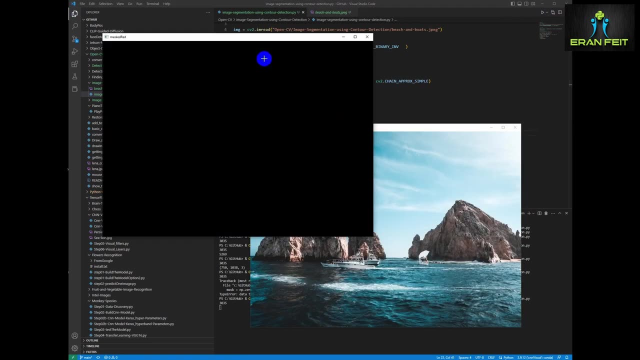 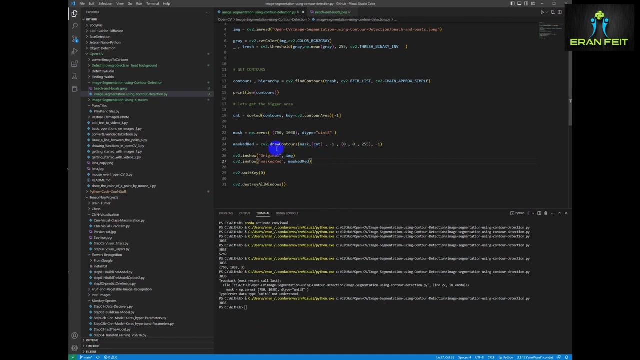 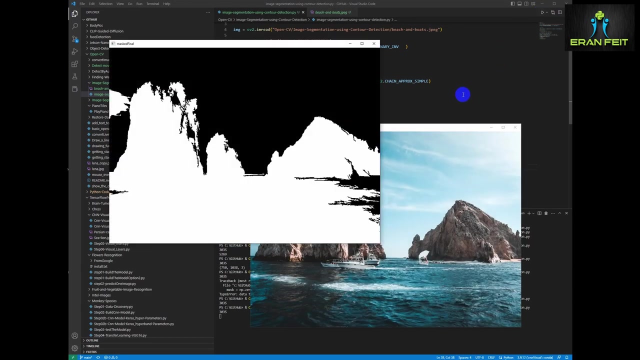 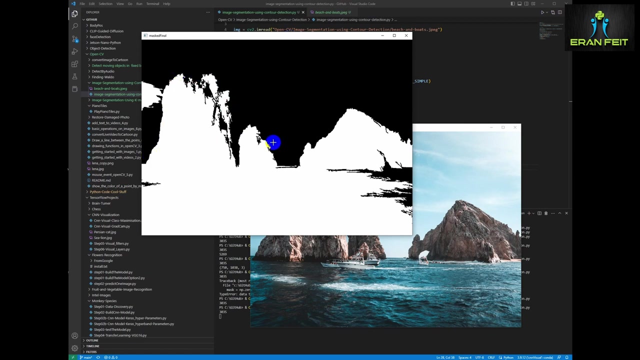 be good enough. if not, we will need- uh, i have a syntax error here. let's fix it. if it will not work, we will try the full channel. so so it's all black. so let's try a different, different approach. let's try it again. okay, that's better. so now we have all the contours, all the relevant contours. 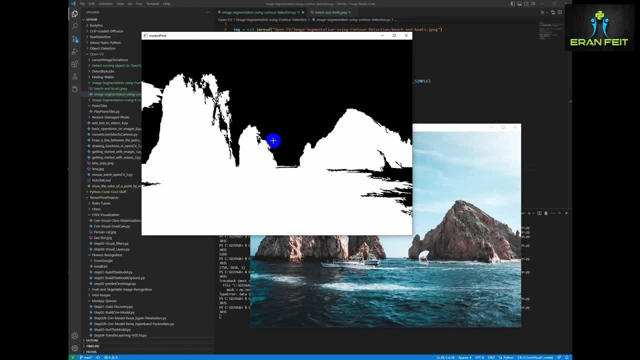 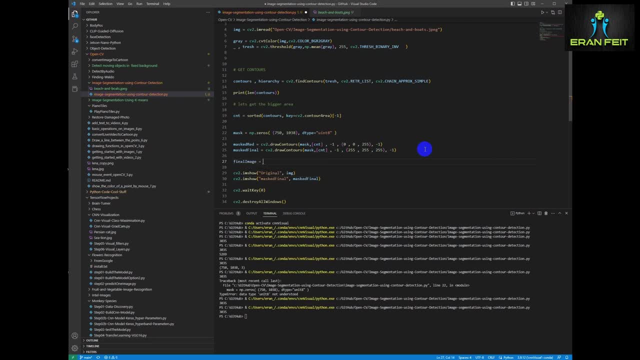 for our segmentation. so now let's merge it with our original image. so the mountains and the sea will be the original image, and the backwards and the forward movement will be the original image. so let's set this right and make sure we have a good contours for our segmentation. so now let's 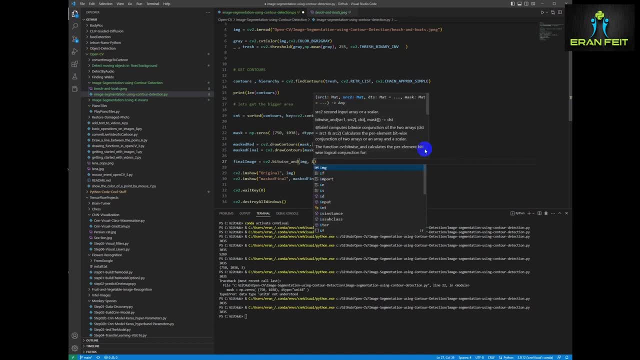 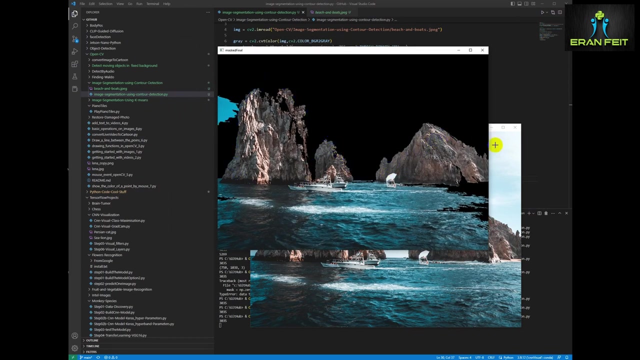 the black background will stay black. so we will use the cv2 bitwise and we will send our image and the mask. now let's display this image. so now you can see we have the mountains and the sea and boats and the background is black. okay, that's. 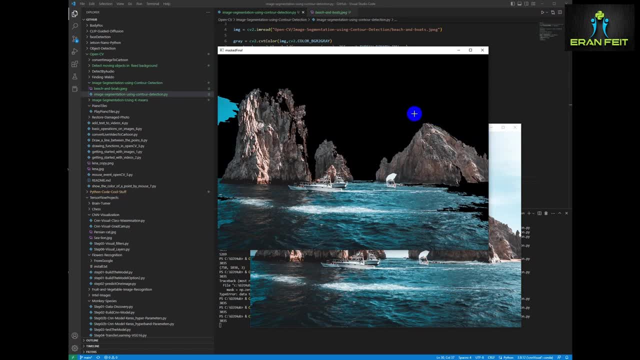 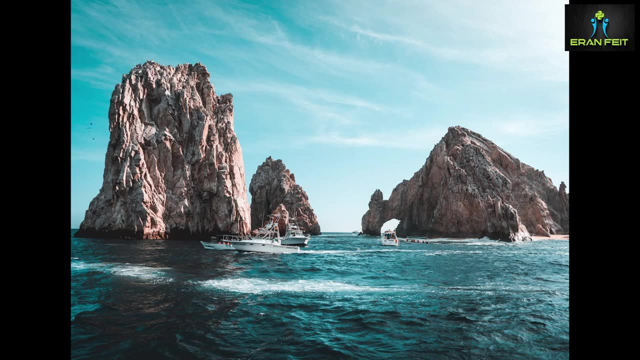 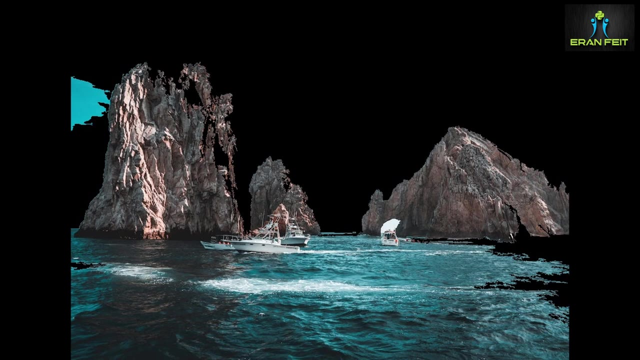 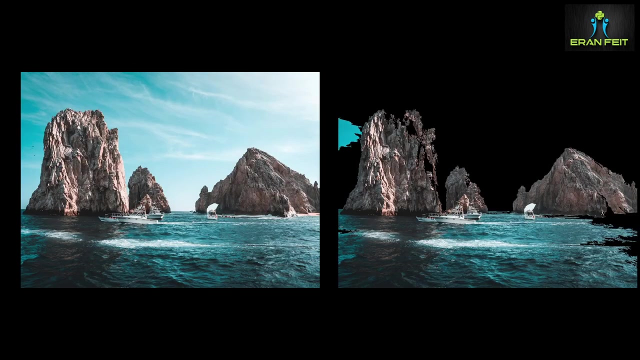 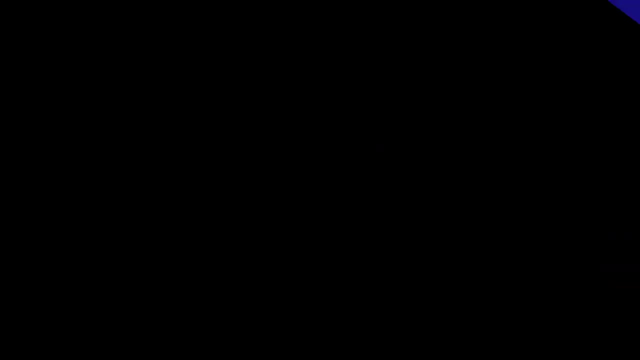 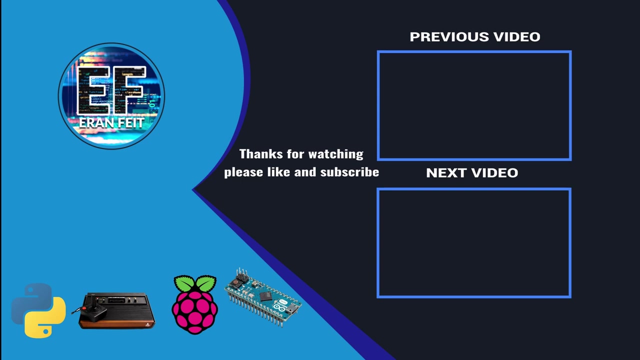 cool. let's enlarge the image and then to see the differences. so this is our original image and this is our segment image. cool. thank you very much. hope you enjoyed this tutorial. you are most welcome to subscribe my channel for the next videos. bye, bye you. 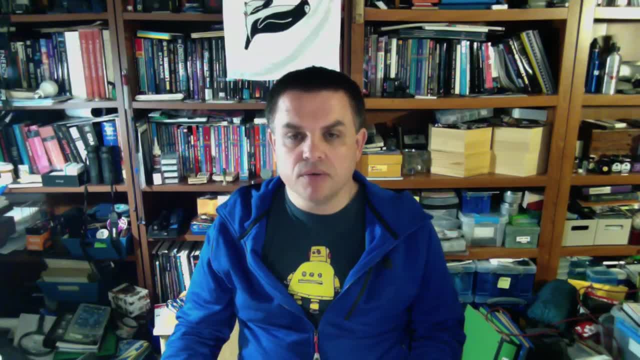 Hi class. this is the first video for the first day of lecture. If you were with us today, we met at our normal class period meeting time so that we could just talk about how the class goes, but all the content in the course is going to be: 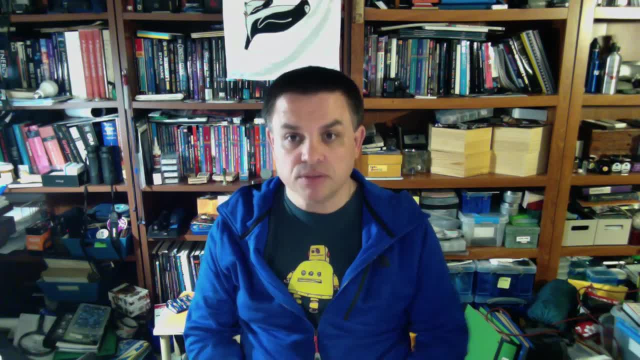 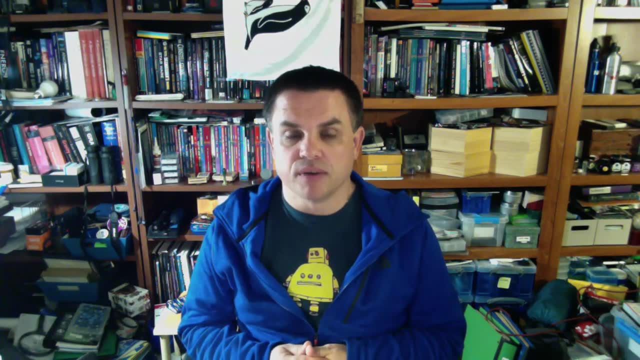 delivered asynchronously. So I'll pre-record lectures, just like this one. I'll post them to the Canvas site so that you can watch them whenever is convenient for you, in whatever situation you find yourself in. Now, as I said in the syllabus and as we talked about in the orientation today, we are 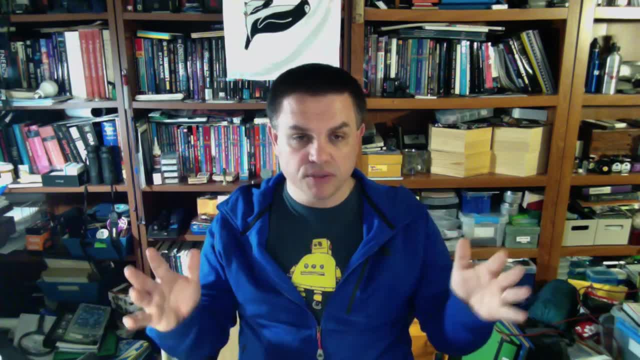 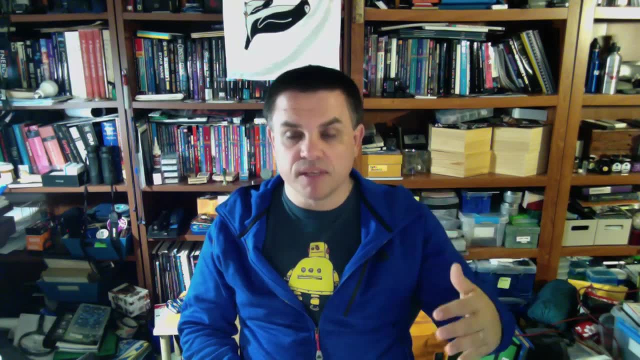 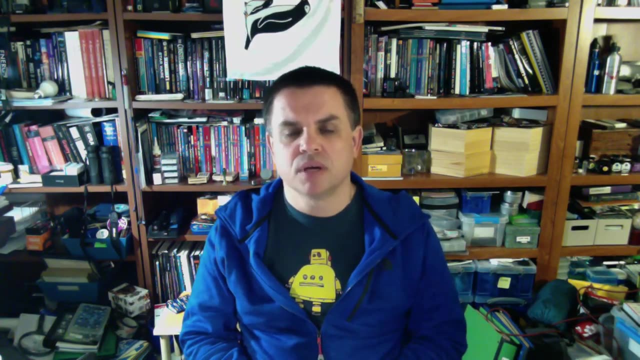 going to not have entire hour-long lectures for you to sit and watch. Instead, I'm going to break them up into little smaller bits, so every lecture will have a couple of different videos for you to watch. They should be short and compact, maybe 10 minutes long, maybe 15 minutes long at most, so that you can